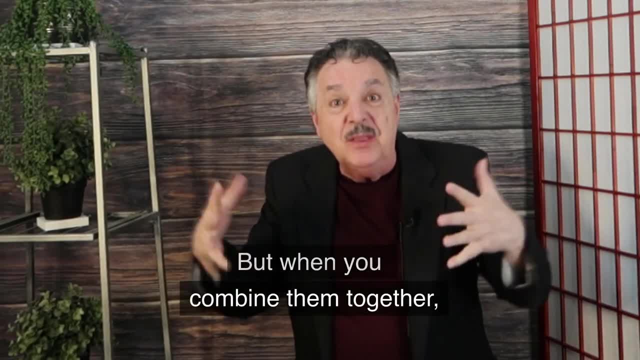 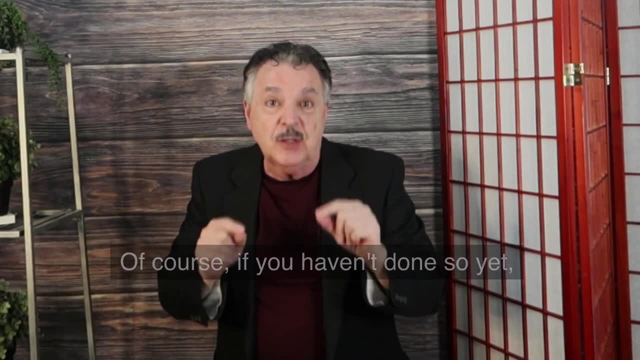 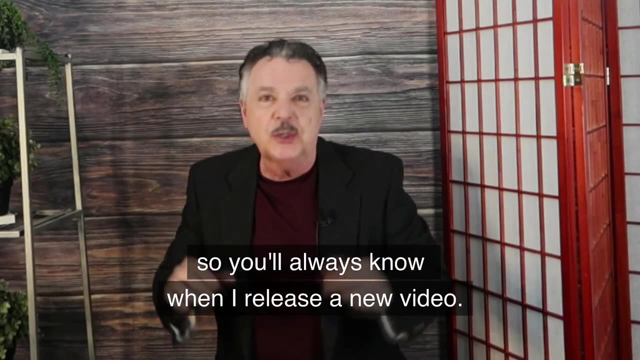 is that big of a deal, But when you combine them together you become a test-taking machine who gets top marks. Of course, if you haven't done so yet, I hope you subscribe with notifications enabled with that little bell icon, so you'll always know when I post a new video. 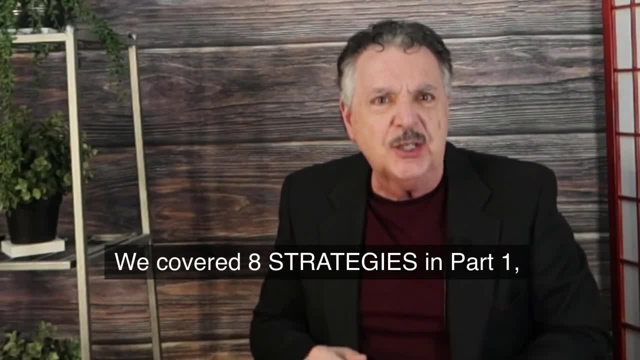 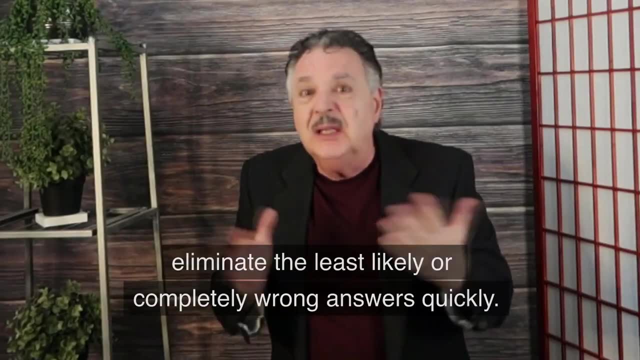 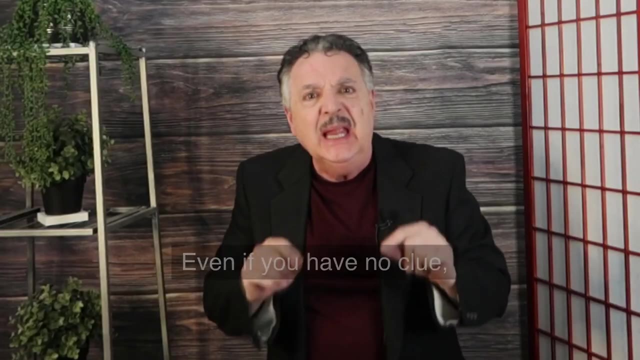 We covered eight strategies in part one, so we'll pick up from there. Number nine: pick the answer that's closest. Eliminate the least likely or completely wrong answers quickly. That will leave you fewer choices to select from, Even if you have no. 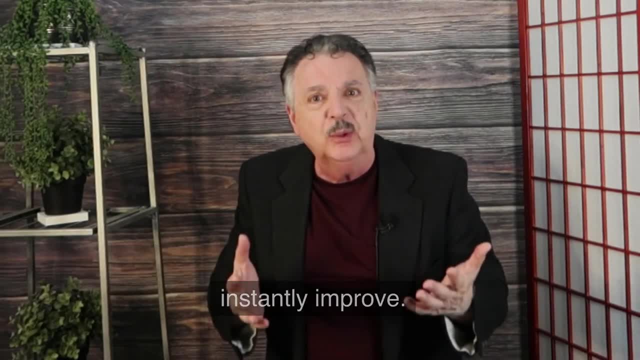 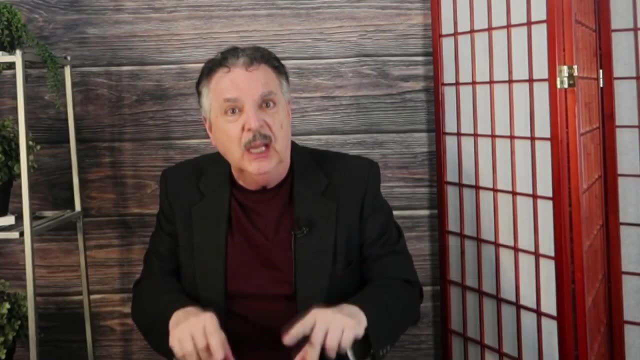 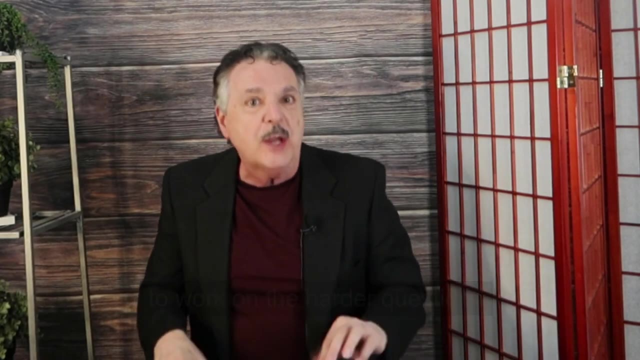 clue, your odds of getting the right answer instantly improve Now. you're probably already doing that now, but pay special attention to this strategy because it can really speed up your progress and give you more time at the end to work on the harder questions or go back over the test to review your answers. Sometimes you'll see a pair of 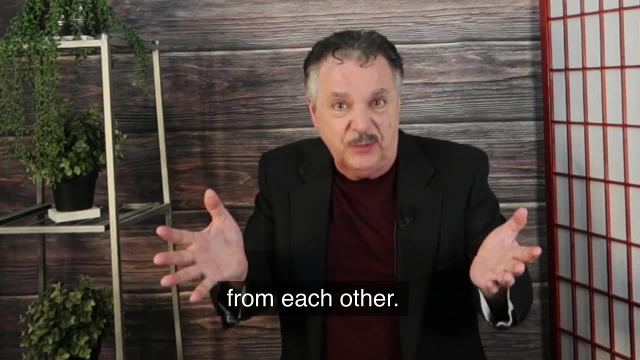 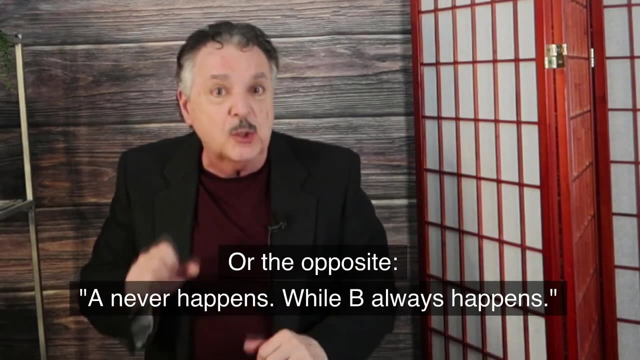 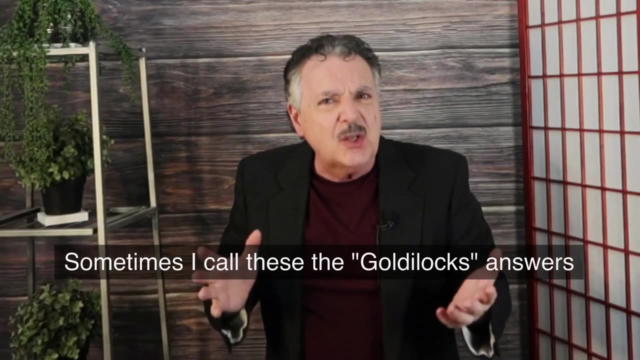 answer choices that say completely opposite things from each other, like A always happens, while B never happens, or the opposite: A never happens, while B always happens. Frequently, one of those choices is the right answer. Sometimes I call these the Goldilocks answers. They happen a lot in math and science exam. 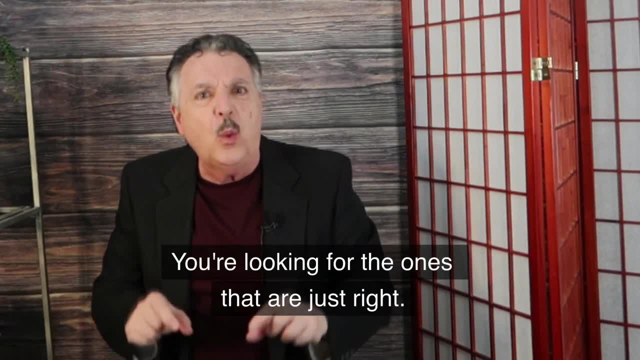 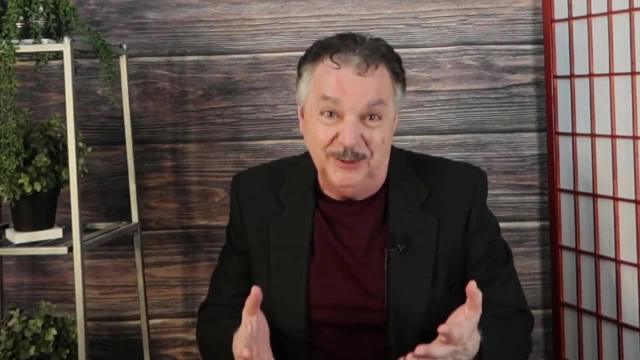 One answer is too high, one is too low. You're looking for the ones that are just right. However, you may be forced to settle for the one that's mostly right, Number ten: pay close attention to the answer choices. Here's another strategy you might. 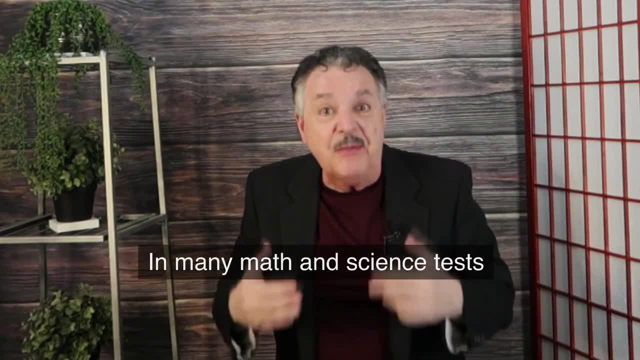 dismiss, but here's why it's included In many math and science tests. you'll see that the answer choices that you're going to pick are the ones that are most likely to be right. Number 10,. pay close attention to the answer choices. Here's another strategy you might dismiss, but here's why it's included In many math and science tests. you'll see that the answer choices 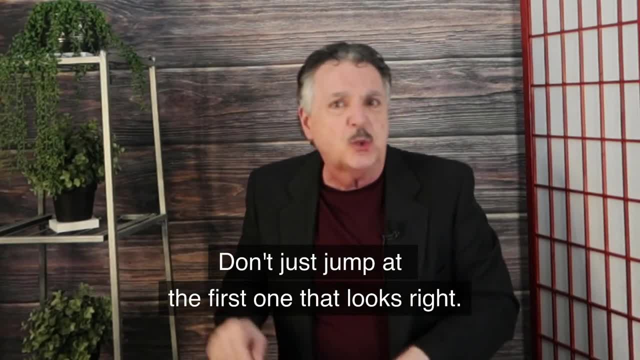 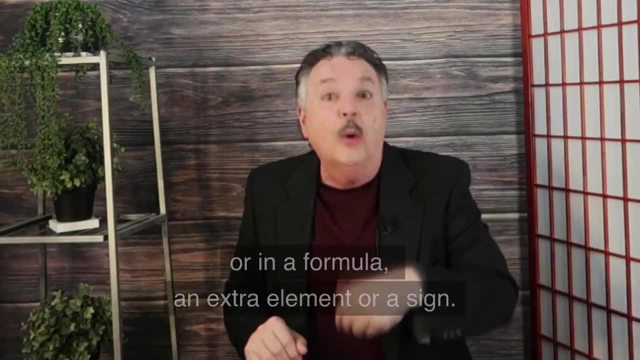 may be very similar to each other. Don't just jump at the first one that looks right. Pay attention to the little things like where a decimal point is, or an extra digit like a zero, or, in a formula, an extra element or a sign. With language classes, you might. 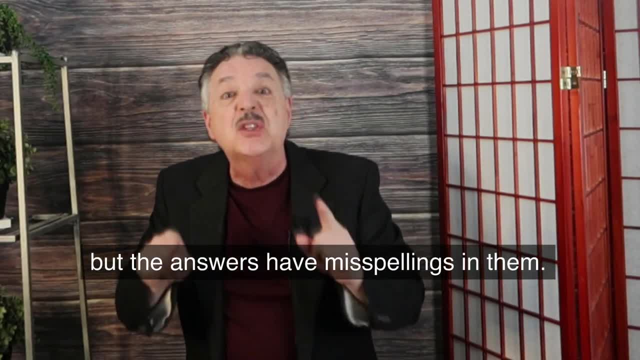 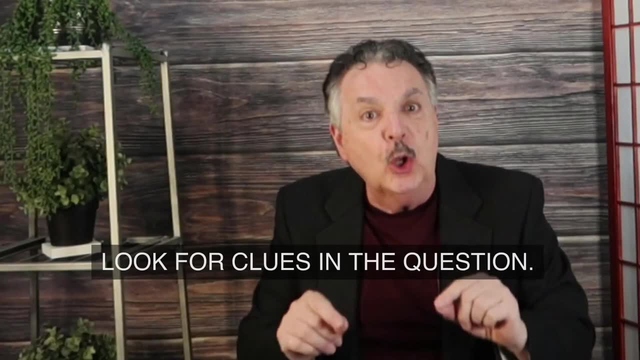 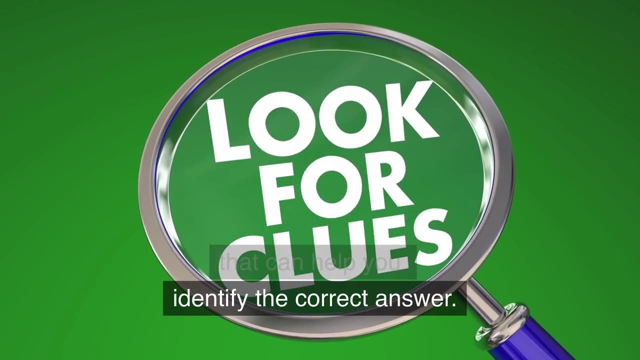 see words that are similar, but the answers have misspellings in them. So, like I said, pay attention to the details. Number 11,: look for clues in the question. Test questions often contain important clues that can help you identify the correct answer. 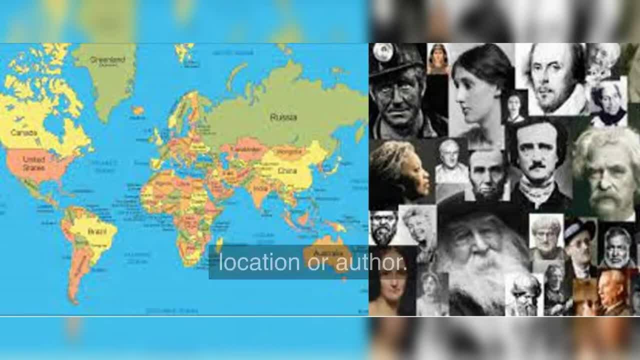 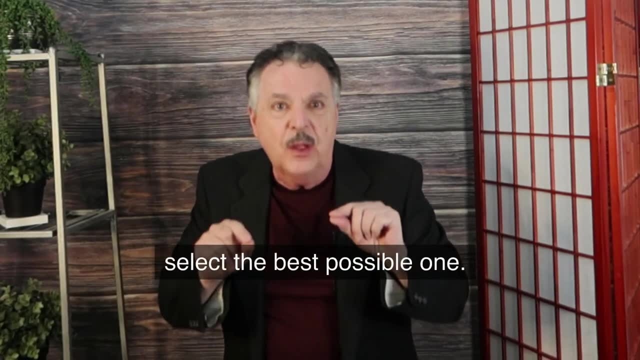 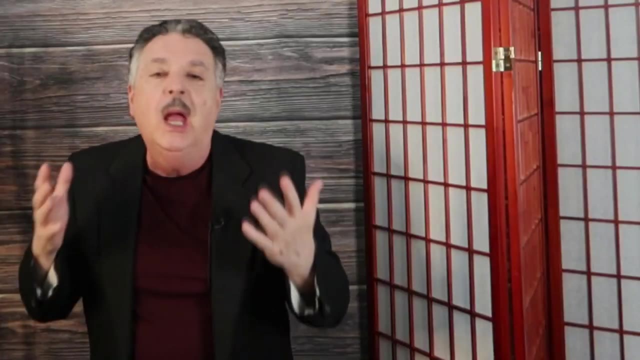 For example, the question might ask about a specific time period, location or author. Paying attention to these clues can help you eliminate incorrect answers and select the best possible one. Number 12,: give the answer your instructor wants. Let's be completely real. Not every teacher or professor is a good one. Some have a political. 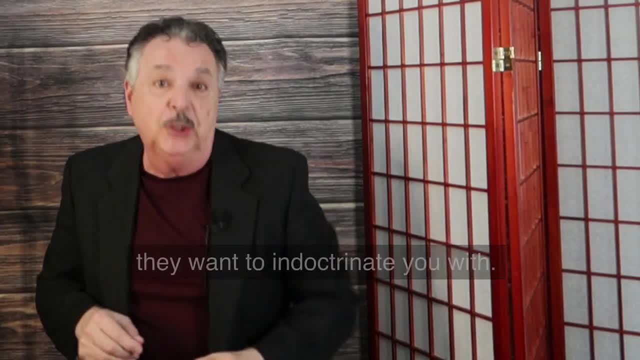 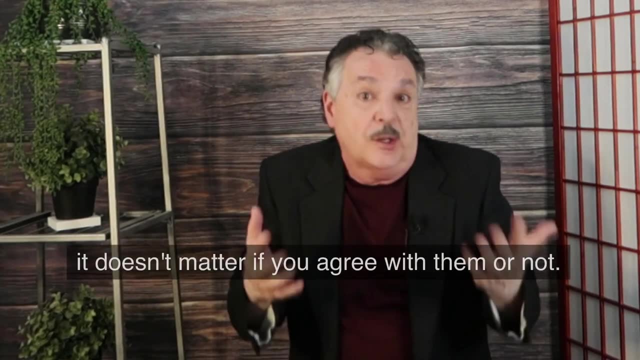 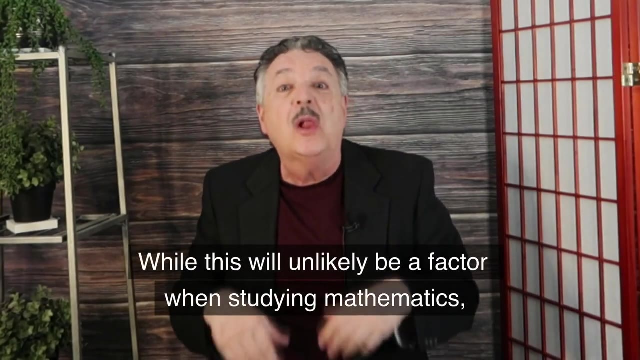 or biased viewpoint they want to indoctrinate you with. If you're just trying to survive that class and come out with a good grade, it doesn't matter if you agree with them or not. Give the answer your instructor wants. While this will unlikely be a factor when studying mathematics, you'll likely be confronted by it in the 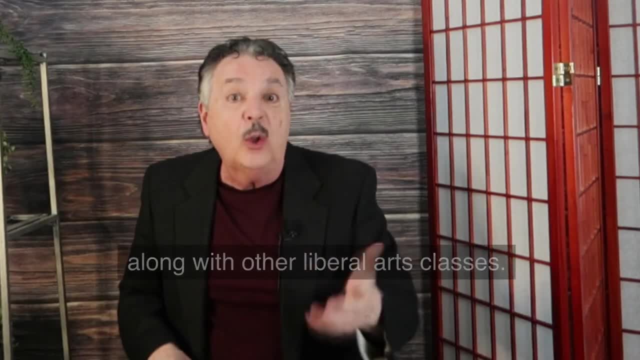 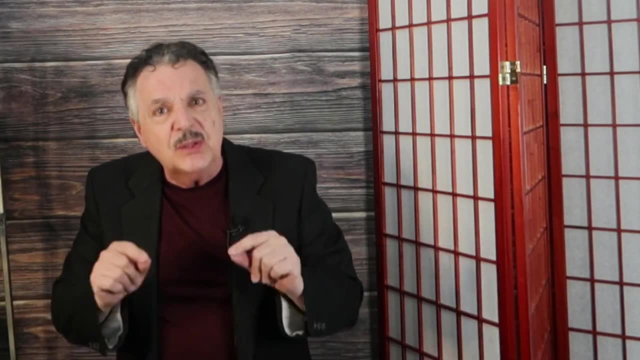 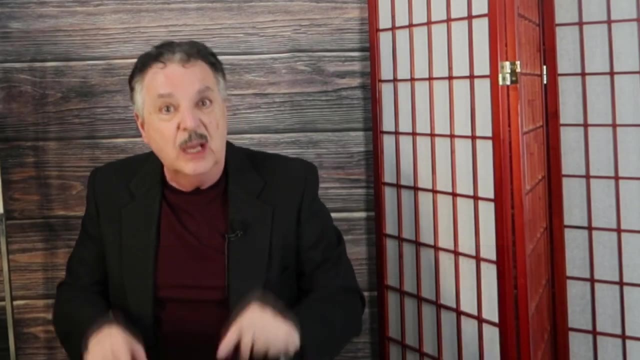 soft sciences like psychology and sociology, along with other liberal arts classes. You may not like what I'm saying, but my only point is that taking an exam is not the time for you to challenge the instructor by espousing your personal beliefs For the sake of getting. 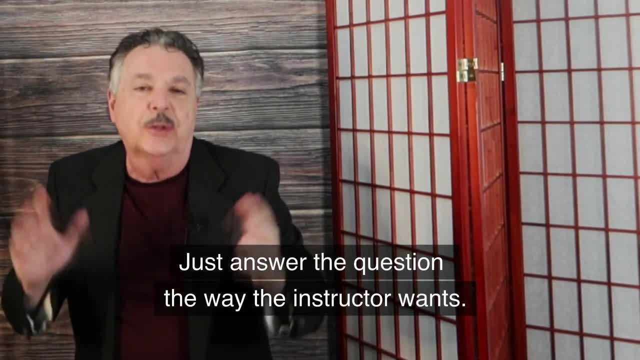 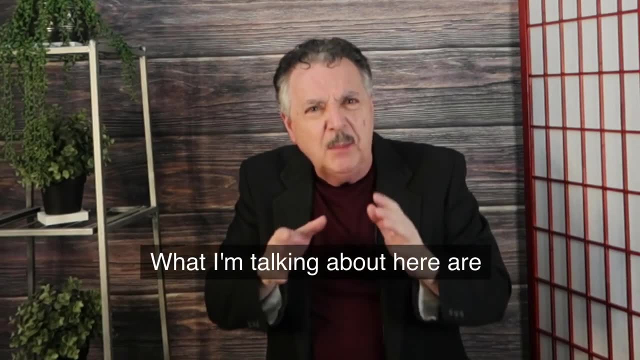 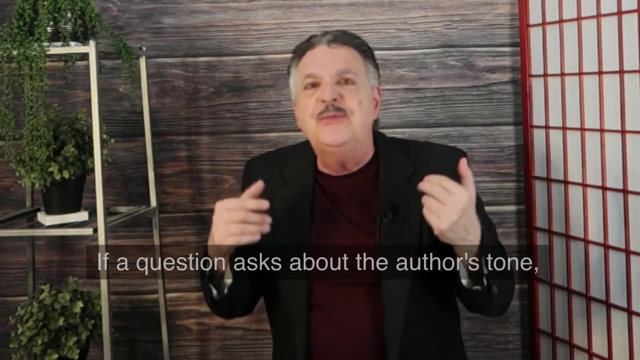 out of there and getting a good grade. just answer the question the way the instructor wants- Number 13,. use context clues. What I'm talking about here are words or phrases in the question that can help you identify the right answer. For example, if a question asks about the author's tone, the answer choices may include: 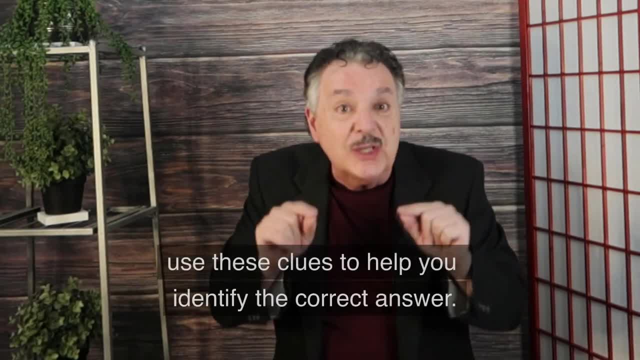 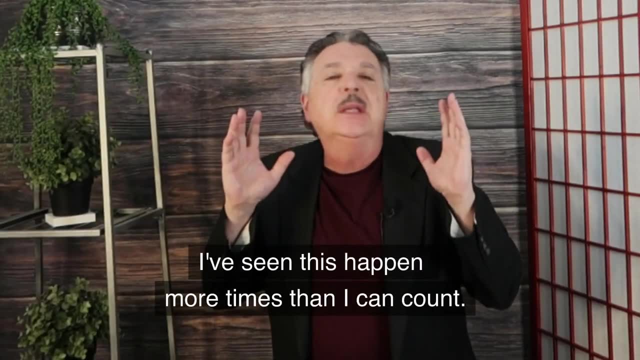 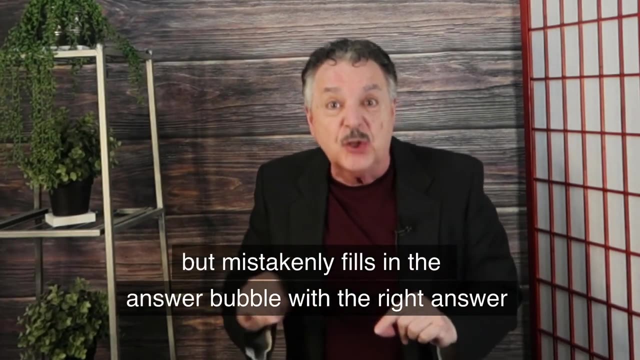 words that describe different tones. Use these clues to help you identify the correct answer. Number 14,. stay organized. I've seen this happen more times than I can count. A student misses one question but mistakenly fills in the answer bubble with the right answer. 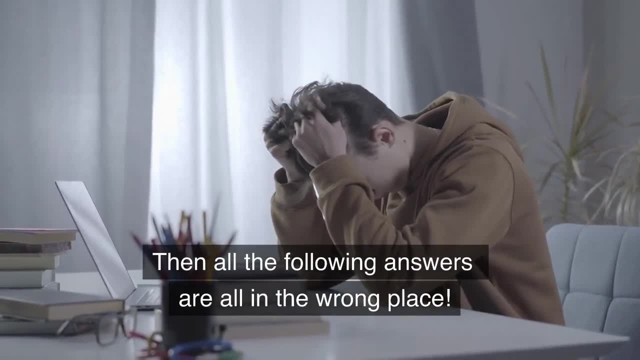 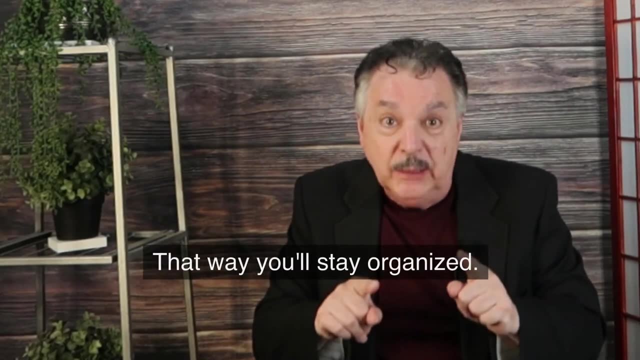 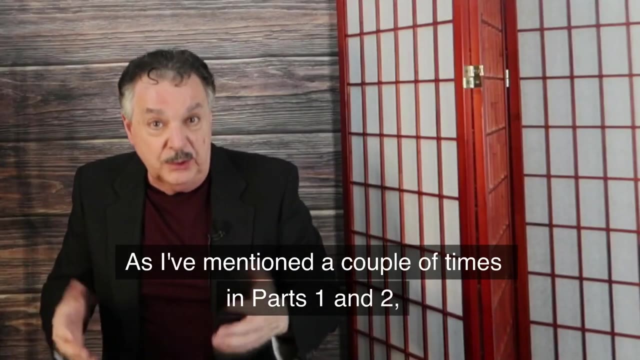 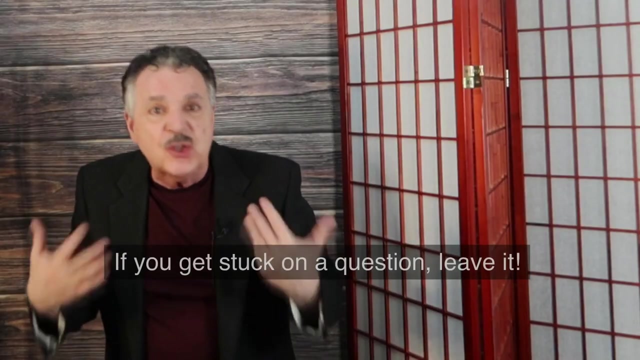 but in the wrong place. Number 15,: manage your time effectively. As I've mentioned a couple of times in parts one and two, good time management is essential for getting top marks. If you get stuck on a question, leave it, Come back to it later, Mark it or make a note of it You want to. 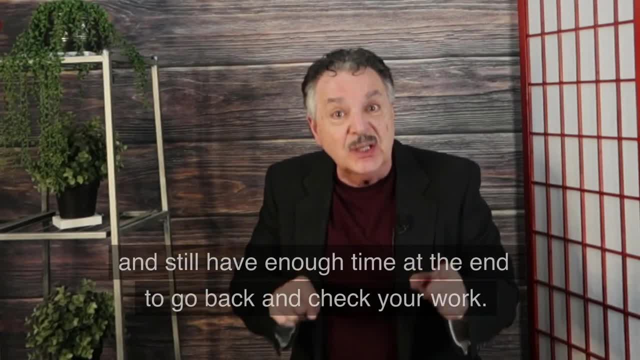 make sure you get through the entire test. Number 15,: manage your time effectively. As I've mentioned a couple of times in parts one and two, good time management is essential for getting top marks. If you get stuck on a question, leave it, Come back to it later, Mark it or make a note of it You want to. 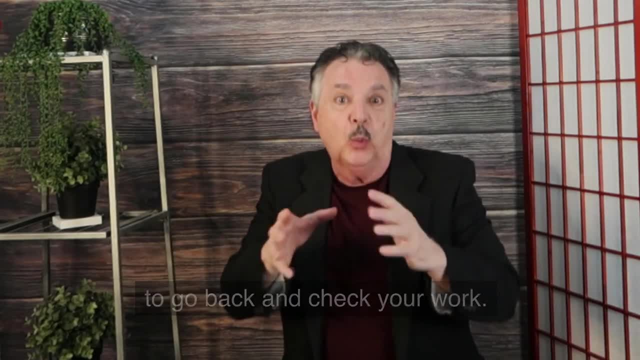 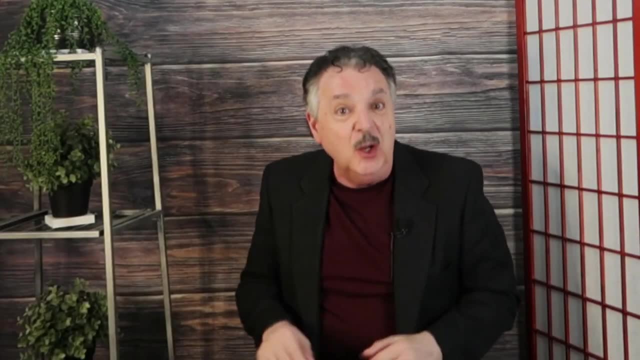 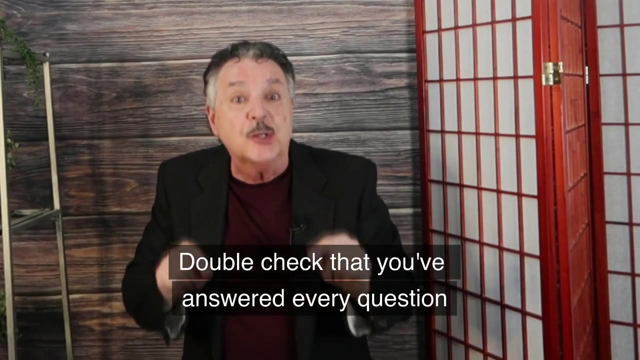 make sure you get through the entire test and still have enough time at the end to go back and check your work. Number 16, review your answers and check your work. No surprise there. We just mentioned it in the previous strategy. After you've answered all the questions, review your answers. Double check that you've answered. 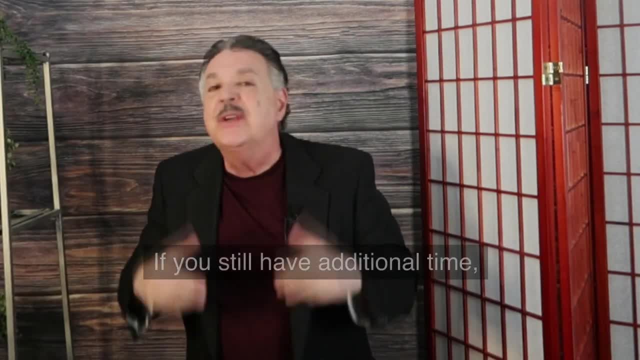 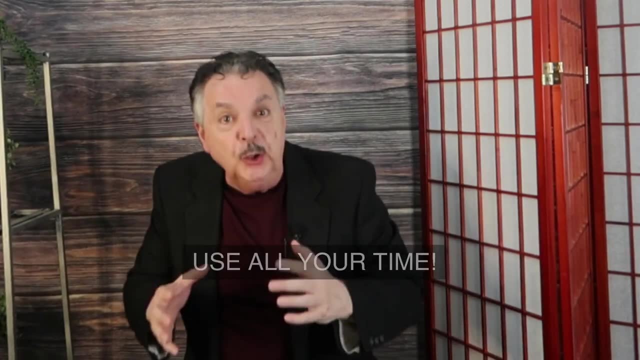 every question and your answers make sense. If you still have additional time, use it to review your answers again. One additional point to this: Use all of your specific answers to compare and half weigh themミー all your time, just because you finished early and even checked your work. 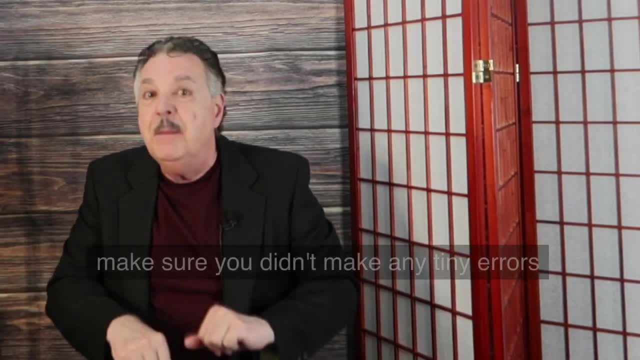 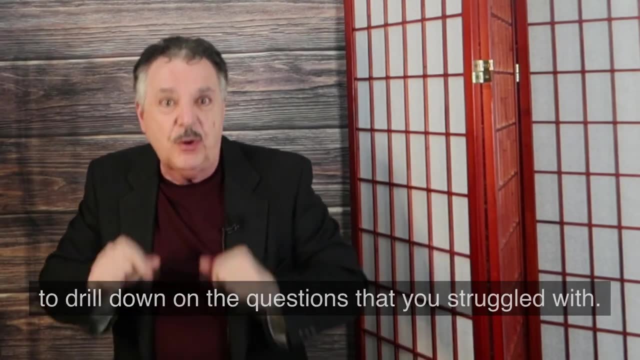 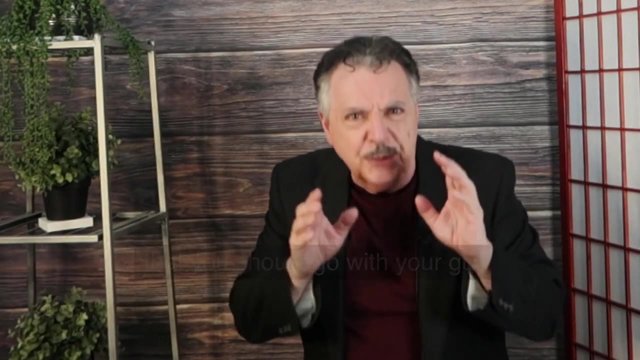 If you still have time, go back over your test again. Make sure you didn't make any tiny errors, Or use your remaining time to drill down on the questions that you struggled with. Now I've got two bonus tips for you. You've probably been told that you should go with your gut, your instinct, on answers. 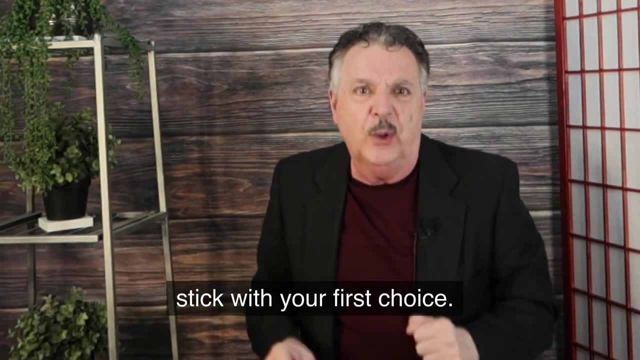 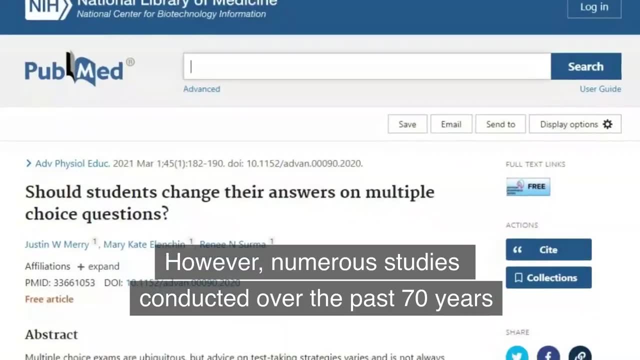 that you're not sure about. You've been told to stick with your first choice. Well, that's good to do with the answers you've got a lot of confidence in. However, numerous studies conducted over the past 70 years have shown that students who 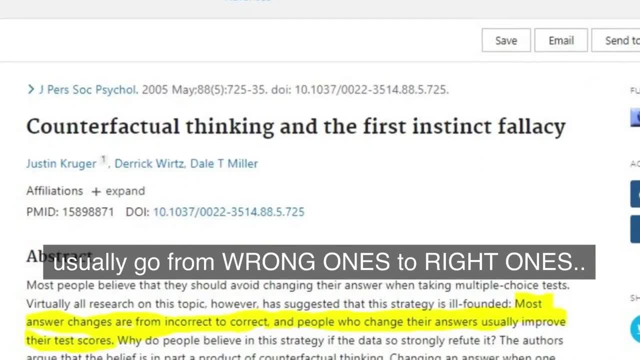 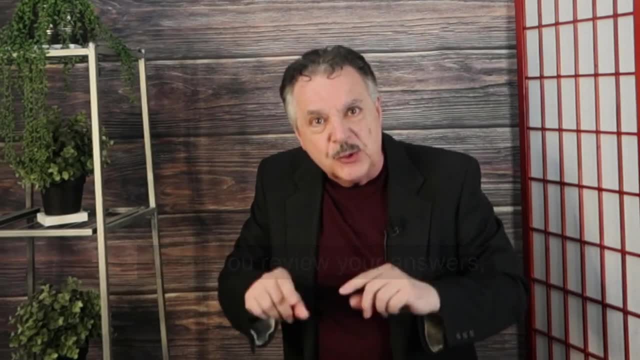 change. their answers usually go from wrong ones to right ones. That's the opposite of what you've been told. But here's the way to do it: When you review your answers, give yourself a mental grade on your level of confidence in that answer. 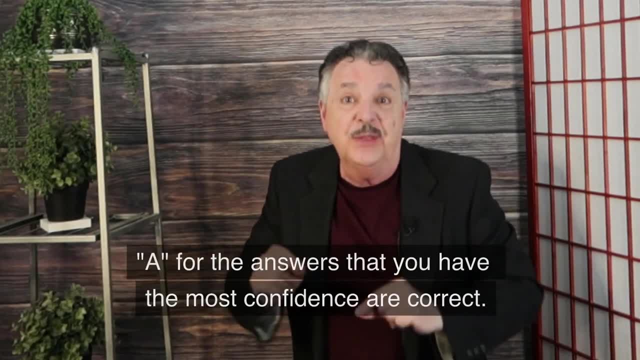 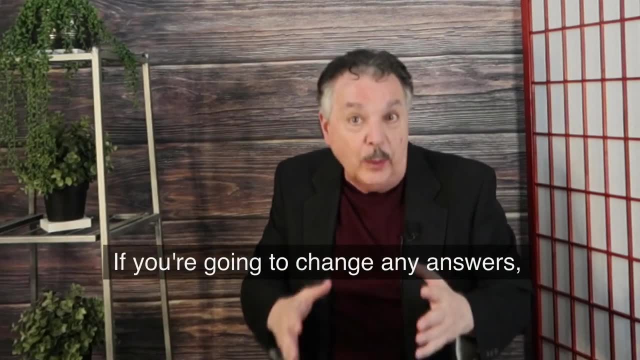 A, B, C, D or F. A for the answers that you have. A for the answers that you have the most confidence are correct. F for the ones you have very little confidence in. If you're going to change any answers, start with the F's.